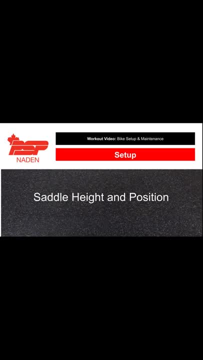 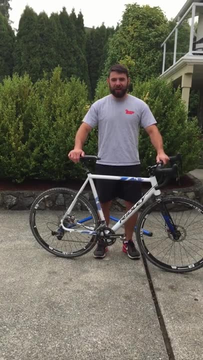 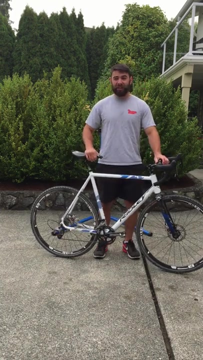 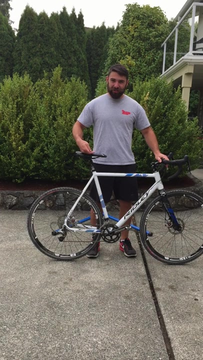 So for setup, we'll be looking at your saddle height, your handlebars and your controls. We'll do this to maximize your efficiency and comfort while riding. So first let's look at saddle height. So we want to make sure your saddle height is the right height for you to maximize. 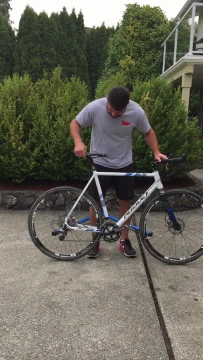 your power use. So we're going to start with the saddle height. So we're going to start with the saddle height. So we're going to get the saddle height. So we're going to get the saddle height from your legs. As you can see, there's a clamp at the bottom of your saddle or seat tube. 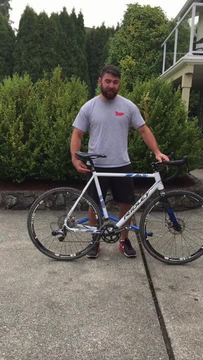 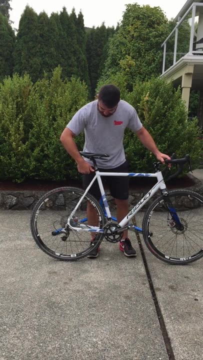 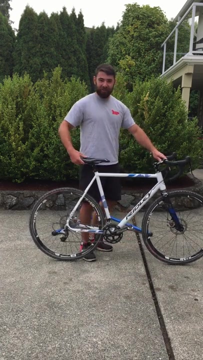 there's two different types. This one here uses a hex key or some have a quick release clamp. If you have a hex key you'll want to put that in turn. it lefty-loosey to adjust. It should be moved nice and freely from here. We're going to raise the saddle up to the top of our hip-bone. 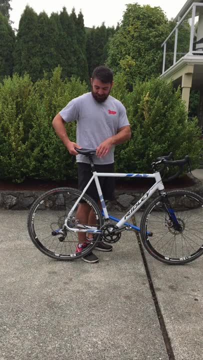 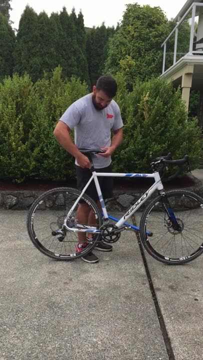 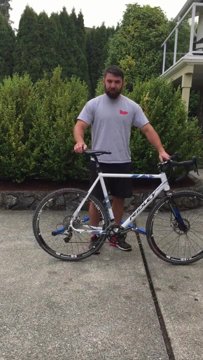 This will give us a good base level to start with. Once you have it there, make sure it's in line with the top tube of your frame and then tighten it down just so it's nice and snug. So now that you have it at that height, let's check to make sure it's the right height for. 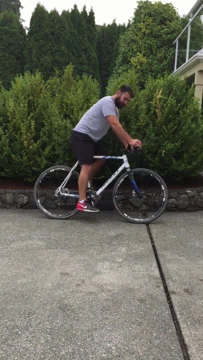 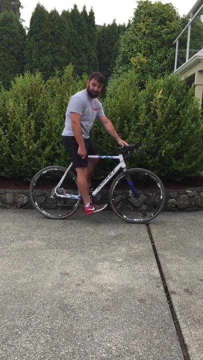 you On your bike. take a seat on the saddle and place your heel on the pedal. With your heel on the pedal, you should have a straight line or a straight leg. That way, when you move your foot into the proper position with the ball of your foot. 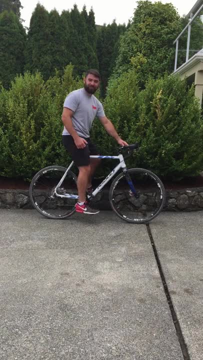 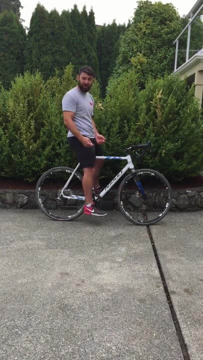 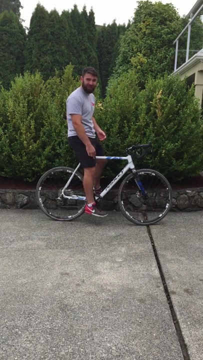 on the pedal, there should be a slight bend in the knee, So it's important to have the right height of your saddle, because if your seat's too low, your knees are going to be up into your chest and not down. It's going to put a lot of strain on your quads and a lot less efficient way to do. 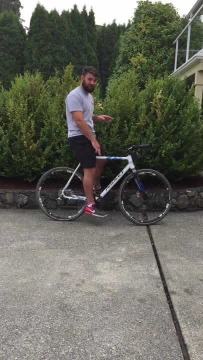 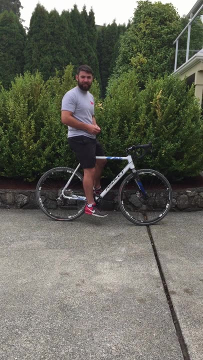 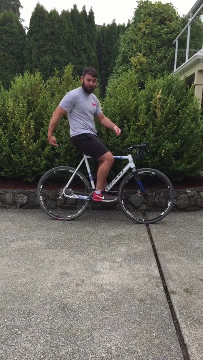 it. Also, if your seat's too high, you're going to be stretching for those pedals and it's going to be awkward and might cause you to fall off balance. So now that we've got the height set, we also want to make sure the position of the saddle 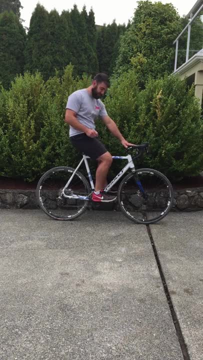 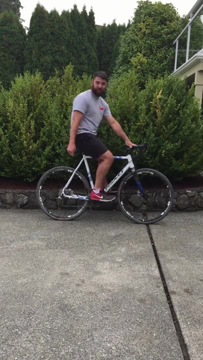 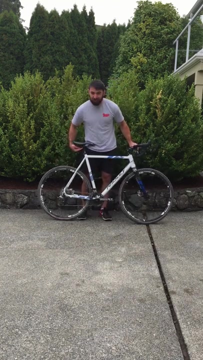 forward and back is in the proper position. The proper position will let your knee be straight. Your knee will be straight over the axle of the pedal when the pedal is parallel to the ground. So to do this, there's two bolts underneath the saddle. 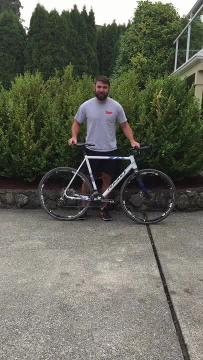 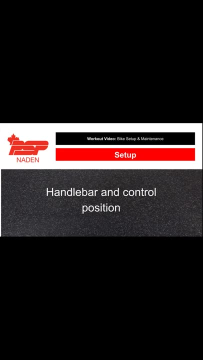 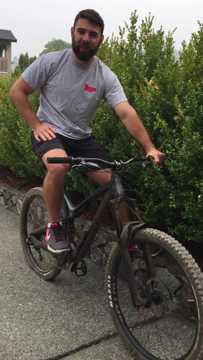 You'll loosen those and then you can adjust it forward or back. So now that we have our saddle in the correct position, we're going to take a seat on the saddle. So, now that we have our saddle in the correct position, let's look at our handlebars. 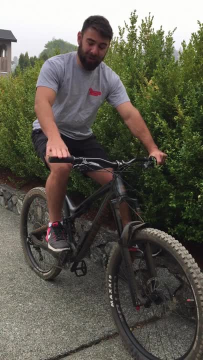 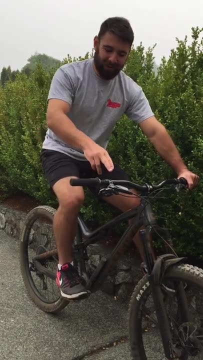 As you can see, I've switched over to a mountain bike which has a straight bar. They use a lot more common type of bar. We'll look at the proper position for this. To start, let's look at our brake levers and their position. 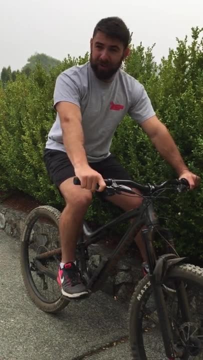 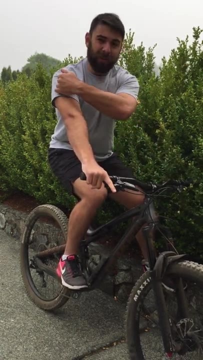 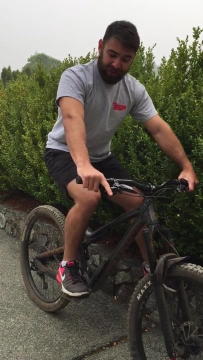 With your hand on the grip, place one or two fingers onto the brake lever, and the brake should be in a position that creates a straight line from your finger all the way up to your wrist. This creates a strong stacked wrist, which provides maximum stability when cycling. 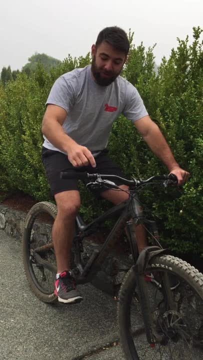 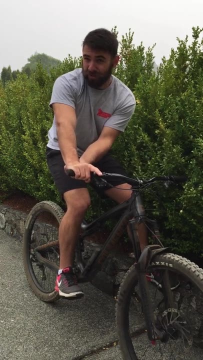 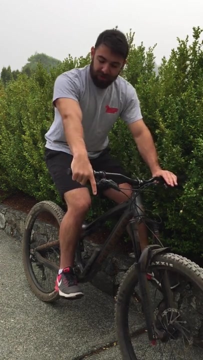 So a couple of things to keep in mind. We don't want our brake levers to be too high, because this will put unwanted tension onto our wrist, which will cause some discomfort during long rides. Also, if our brake lever is too low, this will put a lot of strain on the wrist and thumb. 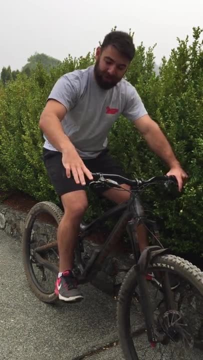 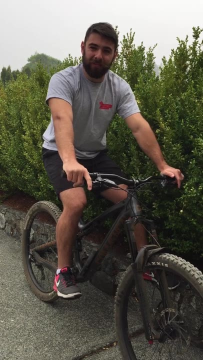 as well. So we want again to keep the brake lever in the right position. We want to have the brake lever in a position where your wrist is stacked and there's a straight line from your finger up to your shoulder, So you don't want to tighten the shifter or breaker too much. 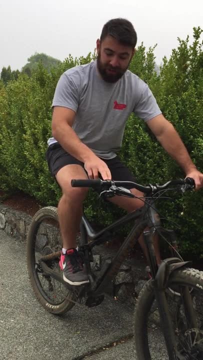 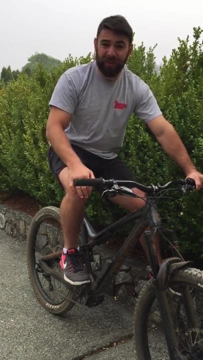 You want it to be a nice snug fit, but not over snug. That way, in the event of a crash, the lever or the shifter will move out of the way instead of breaking. Now that we have the setups done, It's almost time to get out on the road. 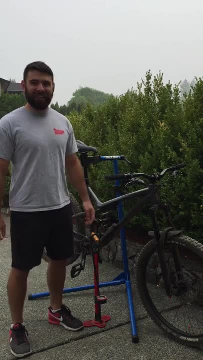 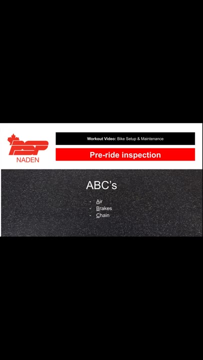 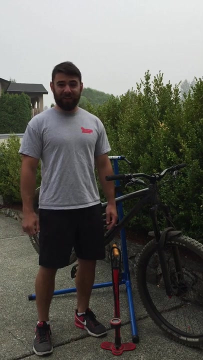 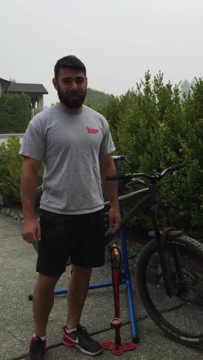 But first let's start with the ABC's of biking. So A stands for air, B stands for brake and C for chain. We'll start with air. So we want to make sure our tires are pumped up to the proper pressure to allow for a more. 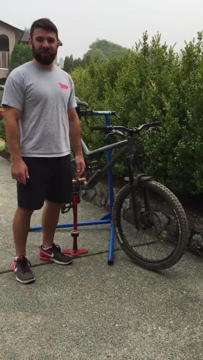 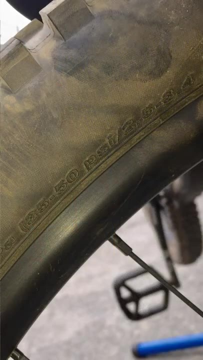 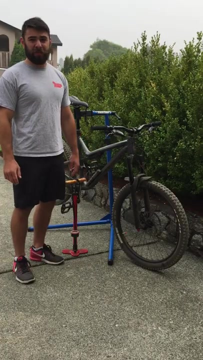 efficient ride. To find the right pressure for your tires, take a look along the sidewall of your tire. They should be imprinted on the side. They will usually give a range for pressures. Higher pressure will be a bit more efficient ride, while lower pressure will be a bit more. 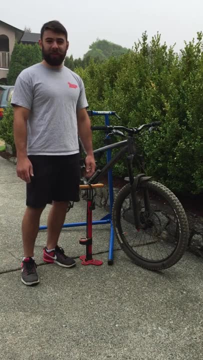 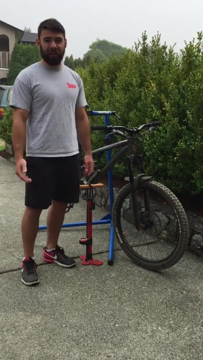 comfortable. Next, we need to know what type of valve your bike needs. There's two main types. There's the older style, which is called Schrader, which is what cars have, and then the Presta valve, which a lot more new bikes have. 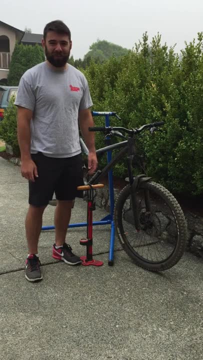 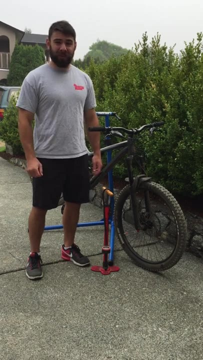 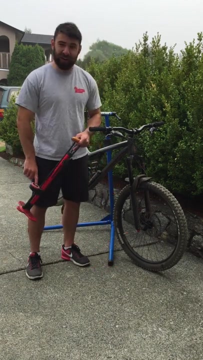 The next step, then, is to grab your pump and inflate your tire to the right pressure. Most pumps these days will have a setting for either type of valve, but make sure you have the proper one. Also, a lot of floor pumps will have a pressure gauge, which will make it a lot easier for. 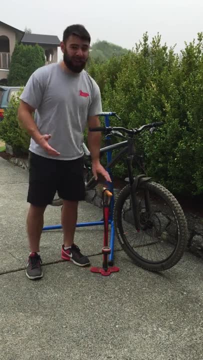 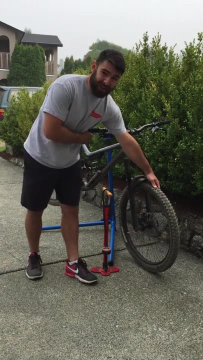 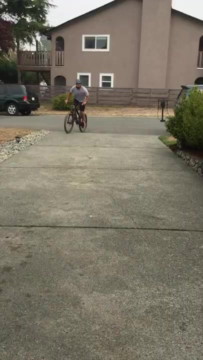 you to get to the right pressure, But if not, you can always use a hand check. If you have a wider tire, Like a mountain bike tire, you should be able to press the tire in slightly with your thumb, while on a road bike or a skinnier tire it should be quite firm. 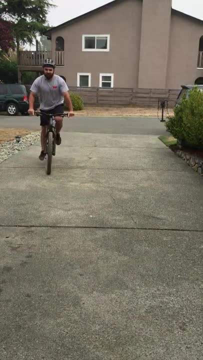 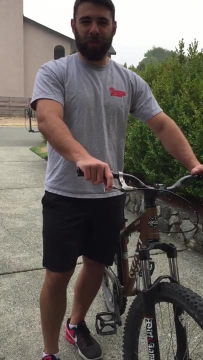 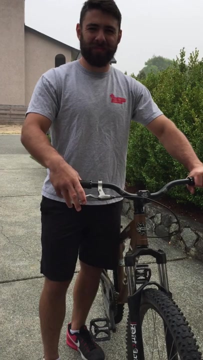 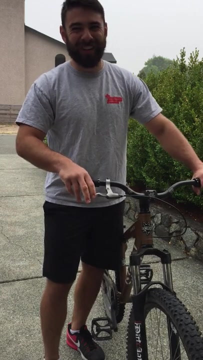 The next step is feet for brakes. We want to make sure your brakes are in good working order so you can maintain control and brake in the case of a flat tire. Do you see anything wrong with this brake I have here Correct? it's too loosey goosey. let's fix that. 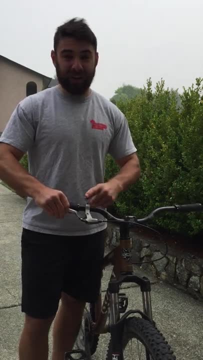 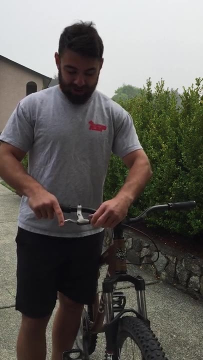 If you're able to pull your brake lever all the way to the handlebar, like I can do here, we can fix that Simply by turning the adjuster knob on the end of the brake lever out. this tightens the cable and provides more bite on the brake. 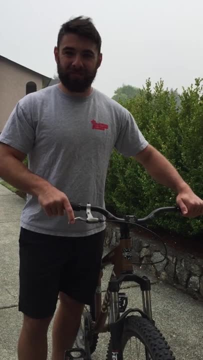 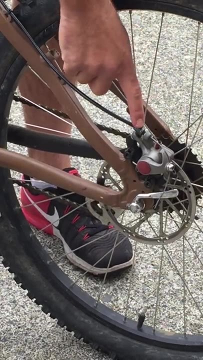 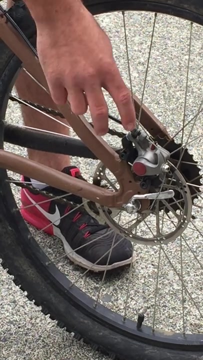 That's it. Thanks for watching. If you've reached the maximum you can on the brake lever, look at the caliper of your brake and use the adjuster knob on there. If that still didn't provide enough tension, reset them back to the lowest they can unscrew. 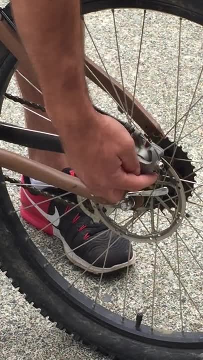 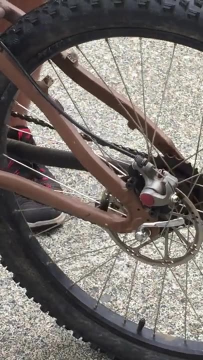 the bolt holding the cable of the brake. pull the cable tight and then reset the bolt. Try again after that. Finally, we're going to look at C for chain. We want to make sure the chain and the gear are all in good working order. so we have. 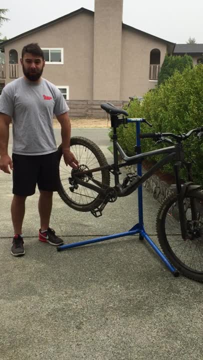 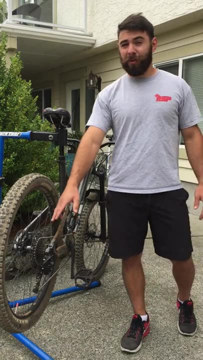 an efficient, smooth ride. We also want to make sure your gears are shifting smoothly and properly to give you a clean, efficient ride. If your chain is skipping or grinding or making any kind of funny noise while you're trying to shift, the simple adjustment will help you to keep the gear in place. 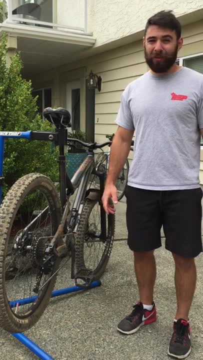 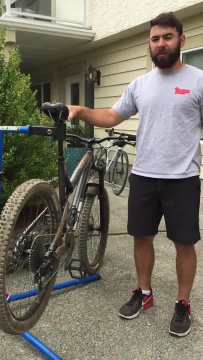 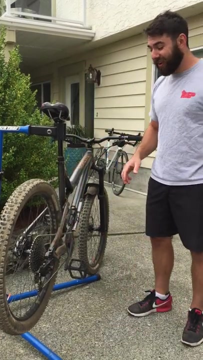 If your chain is moving, you can use the shift knob to shift the gear. That's it. Thanks for watching. See you next time. Bye. So on most new bikes, the cable which controls the derailleur will tend to stretch. It's bound to happen for everyone. so to help alleviate the problem, use the adjuster knob. 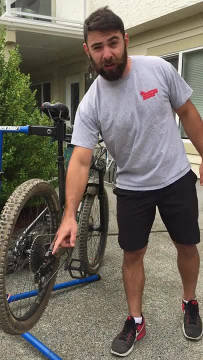 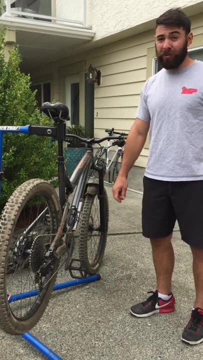 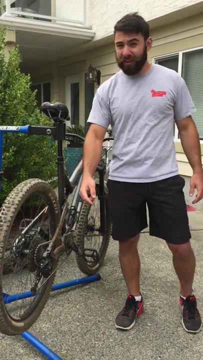 either on the shifter or on the derailleur itself, turning it counterclockwise a quarter turn at a time until you get a clean, smooth shift. If your bike is having trouble shifting down in the gears, your cable is too tight. 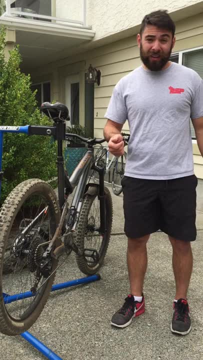 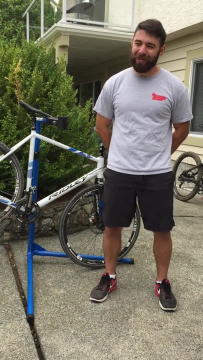 In that case, turn the adjuster knob clockwise a quarter turn at a time until it shifts smoothly. Now that we have the ABCs done, it's time to get out there and ride. But guess what? You've got a flat tire. 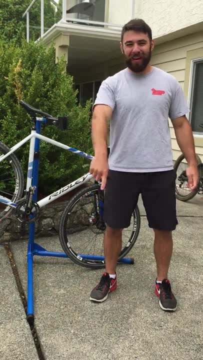 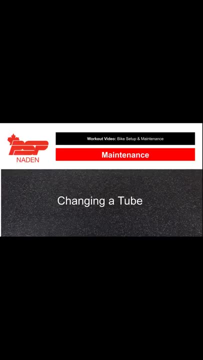 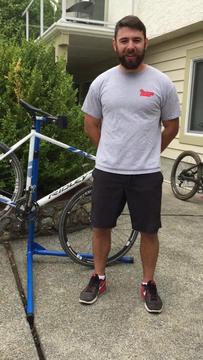 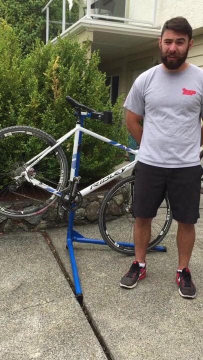 No one knows how it happens, but it's bound to happen. I'm here to show you how to change that too. Welcome to the next section: bike maintenance. So to start, you might need a few tools for this. One that will make your life easier is tire levers. 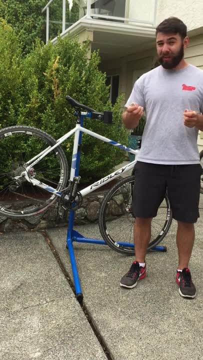 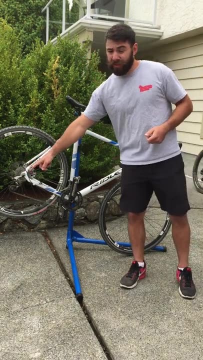 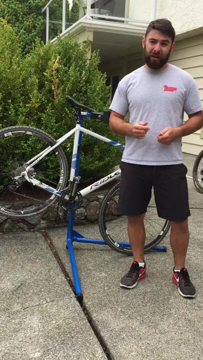 You can get these in either metal or plastic. Plastic will be a little bit more friendly on your rims, Depending on your bike. you might have a quick release For your wheels, which comes in handy, But if not, you might need a certain open-ended wrench or hex key. 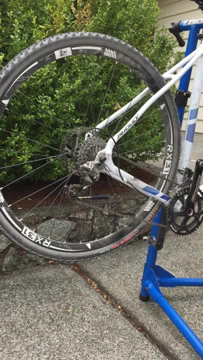 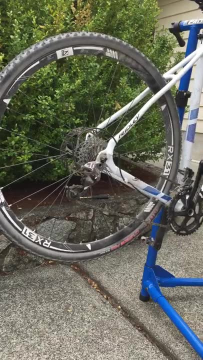 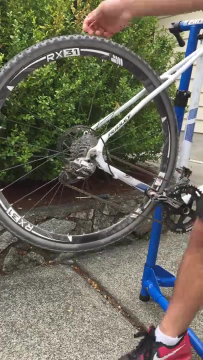 So I'll be demonstrating how to remove your back wheel, because this is the harder one. Front tire is much easier to remove. To start, we're going to downshift to your lowest gear. From there you'll either undo the bolt. 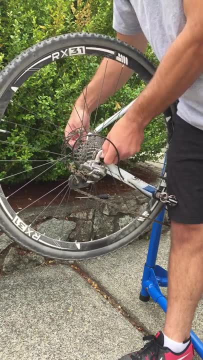 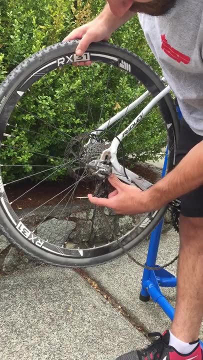 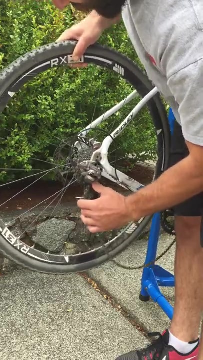 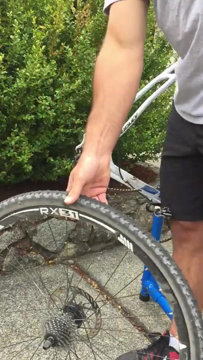 or wrench, or the quick release. Unscrew it slightly or all the way, if your bike requires it, Pull the derailleur hanger out of the way And drop your tire wheel off. As easy as that. Now your back wheel is removed. 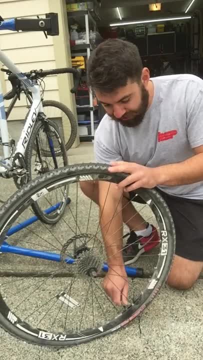 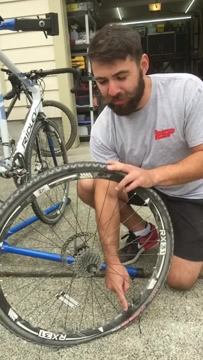 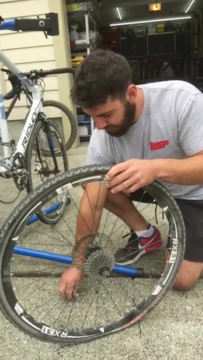 So now that you've got the wheel off, we're going to remove the cap, Undo the core and empty out any remaining air from the wheel. Once all the air has removed, you can grab your tire levers, Stick them in under the tire. 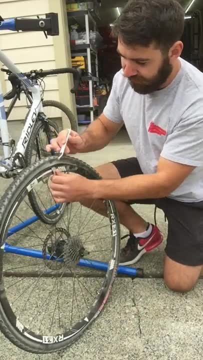 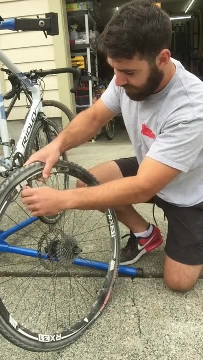 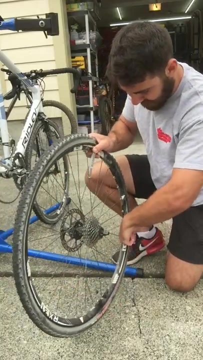 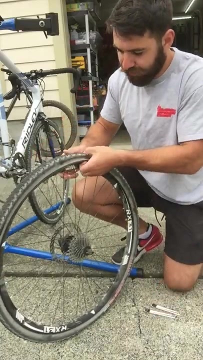 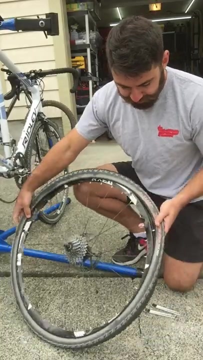 And pull the bead out of the rim. Then you can work your way around until half the tire is off, the one half of the rim. From there, find where the stem of your valve is, Pull the old tube out And remove the old tube. 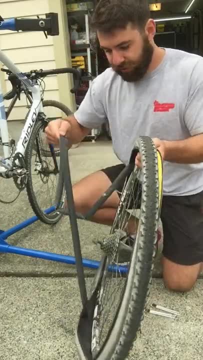 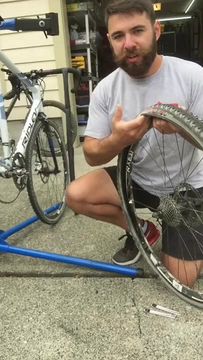 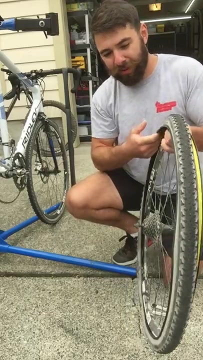 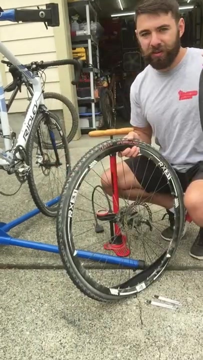 And remove the tube. Now check to make sure that your hand on the inside of the tire is like nothing sharp That will cause your second puncture. You can also check the inside of the rim for the same thing. So next, grab your new tube. 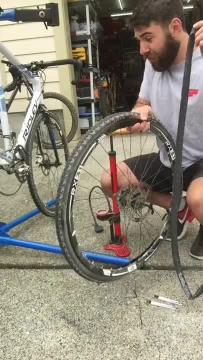 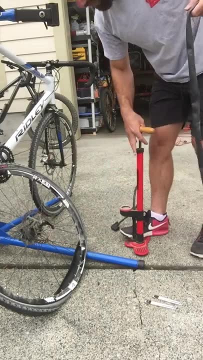 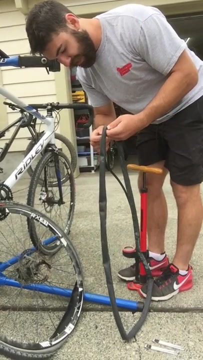 For the purpose of this demo, I'm going to be using the same tube, because it was still good. We want to inflate it slightly, Which will make it easier for us to install it. So grab your pump, Insert the valve And just inflate it a little bit. 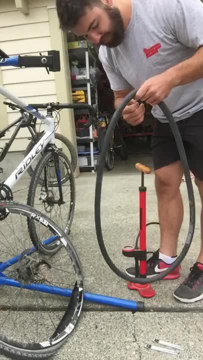 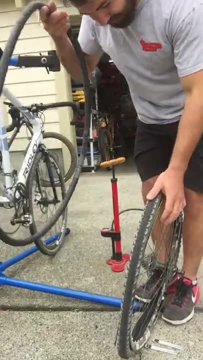 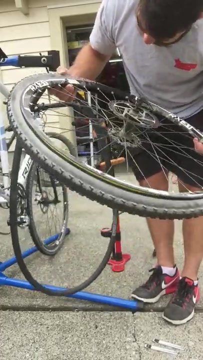 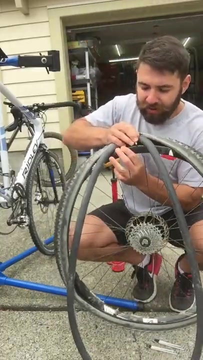 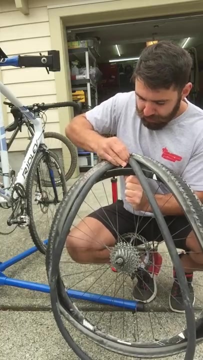 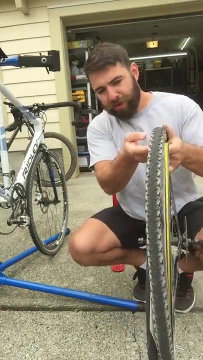 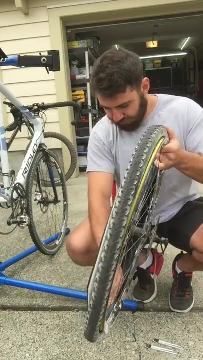 One or two pumps. Next, grab your wheel again, Find the hole in the rim for the valve And push the valve up And then through the hole in the rim. Once that's through, push your tube back into the tire All the way around. 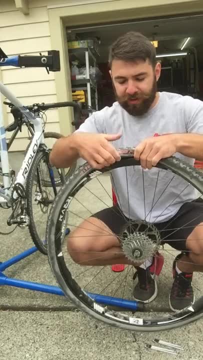 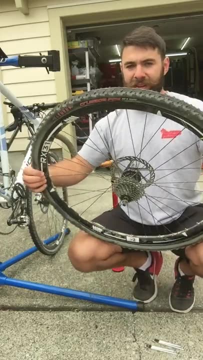 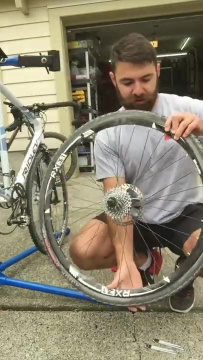 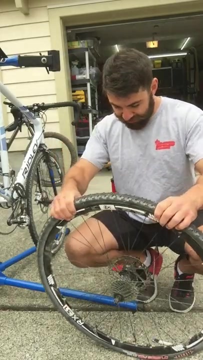 And then push the bead of the tire back into the rim. I like to work my way around with both hands at the same time, And once you get close together it might be a little trickier, So you might need your levers to put it back. 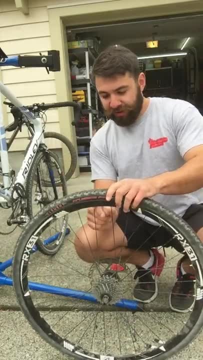 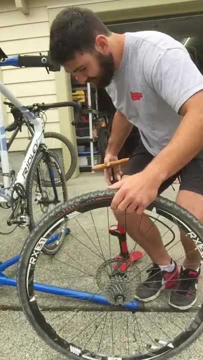 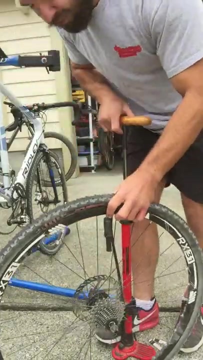 Now make sure you find the stem And make sure it's coming out at a straight angle And not off on an angle or anything at all. Grab your pump And then push the valve back into the tire And re-inflate the tire. 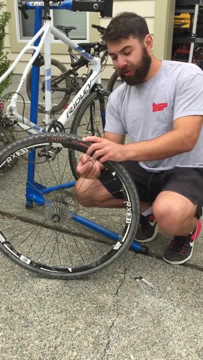 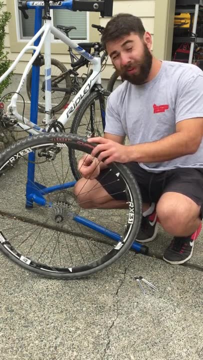 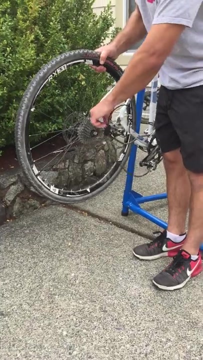 So, now that your tire is pumped up, Make sure you screw the valve core back in. If you have a Presta valve, Put it on the cap And we can reinstall the tire. Grab your tire, Make sure you have it on the right side. 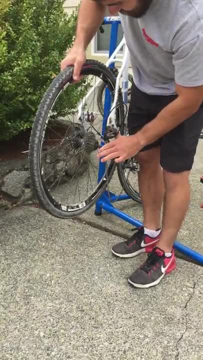 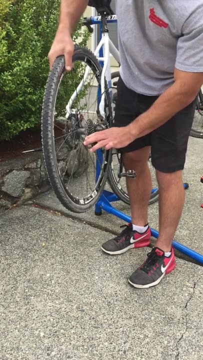 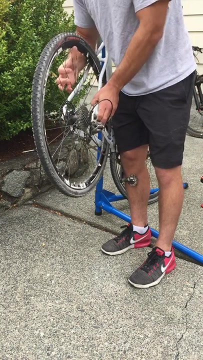 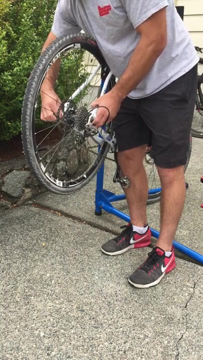 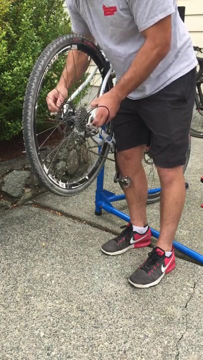 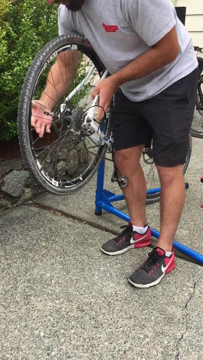 Push the derailleur down, Hooking the chain onto the bottom gear of your cassette, And pull the tire into place Or the wheel into place. Next, tighten up the axle again And finally, if you have a quick release, Clog that up. 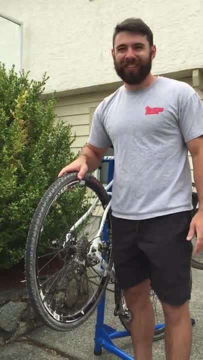 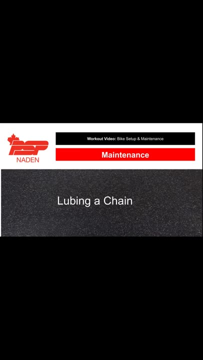 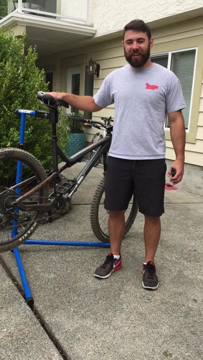 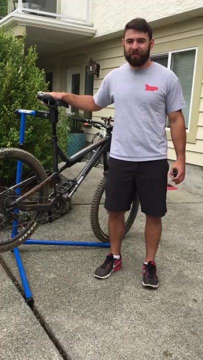 And there you go: You've changed a tire. Next, we're going to look at lubing the chain, Which will help prevent wear on our drivetrain And create a smooth and efficient shift. To start, it's always best to lube a chain when it's clean and dry. 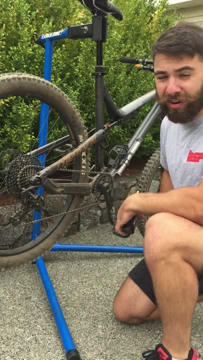 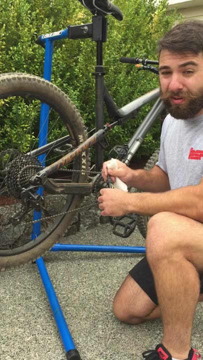 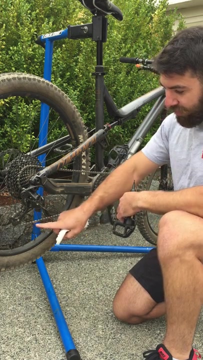 So give your chain a quick wash And dry it off, And then we can start. Any bike shop will carry a selection of lube. Go with what they recommend for your conditions. To start, I like to start On our master link. 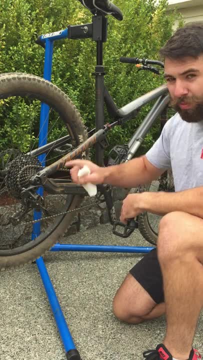 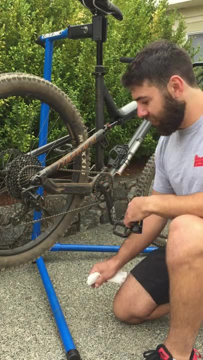 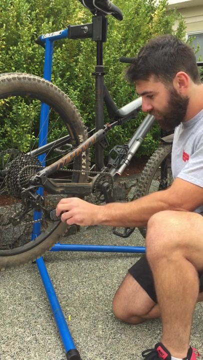 Which is just so you know when you've done the full chain. Most chains will have this, And it's just a special connection point That makes it easier to connect From there. we're going to put one drop of lube on each roller of the chain. 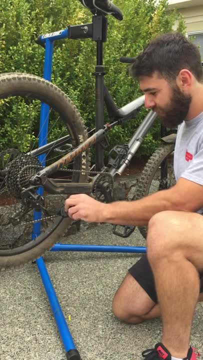 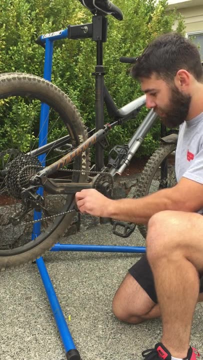 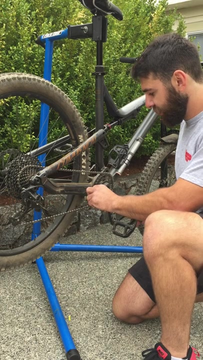 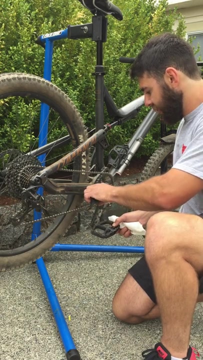 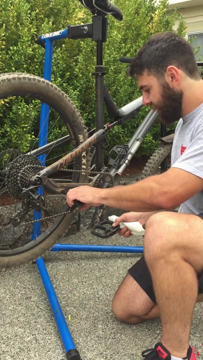 This is a bit of a tedious process, But it's worth it. Once you reach the end, You can cycle through And work your way around the full chain. If you like a little bit speedier process, You can actually keep the bottle squeezed. 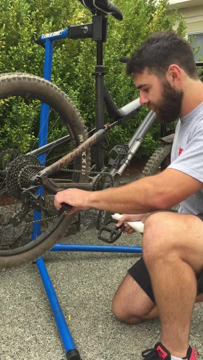 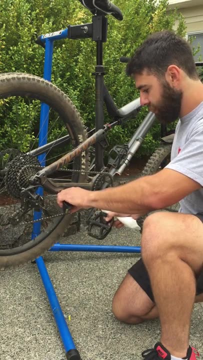 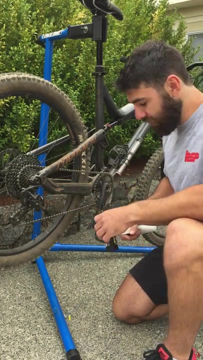 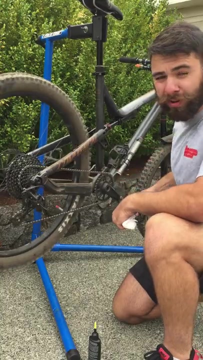 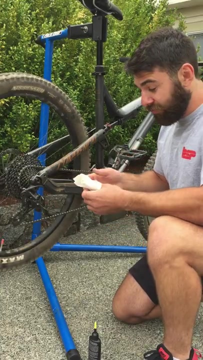 And cycle through Until you reach all the way around. Once you've reached back to your master link, Give your bike a few pedal strokes, Just so the lube can work its way into each roller. Once you've done that, Grab a rag or paper towel. 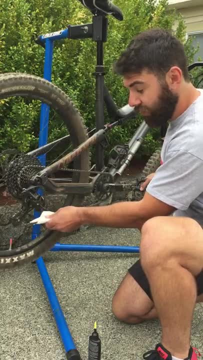 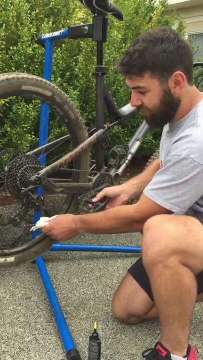 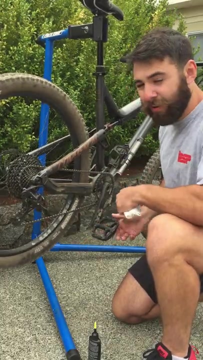 And we're going to wipe off any excess lube. Any excess lube will collect unnecessary dirt and grime in there And cause your chain to creak And inefficient shifts. Once you've done that, You've got a lube chain. 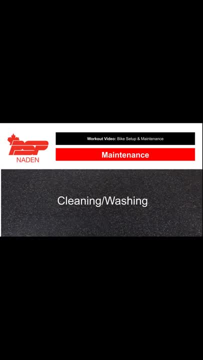 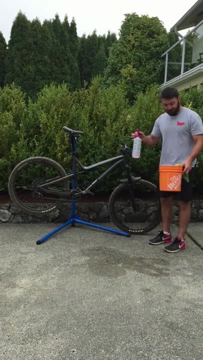 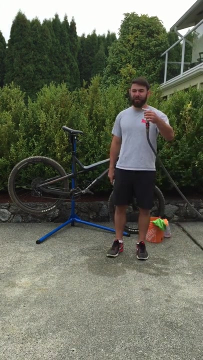 And you're ready to go. The chain bike is a fast bike, So let's look at how we can clean it. A few things you'll need. You can bike wash A variety of rags And brushes. You'll also need a hose. 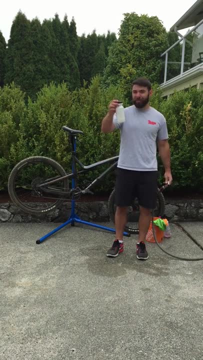 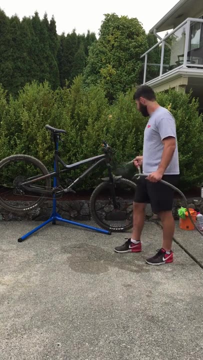 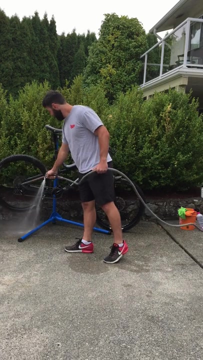 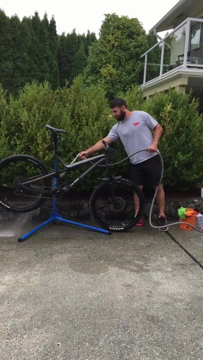 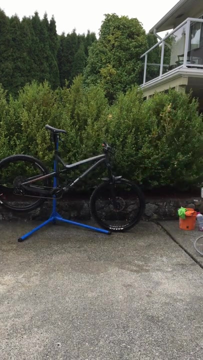 But if you don't have one, No problem, You can also use a water bottle. First step to washing your bike Is giving it a spray. This will help loosen up any of the dirt. Next we'll grab our cleaner And give the whole bike a spray down. 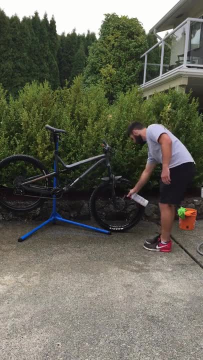 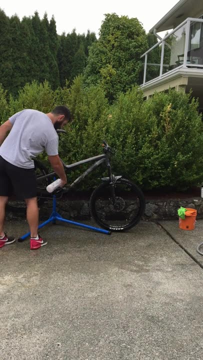 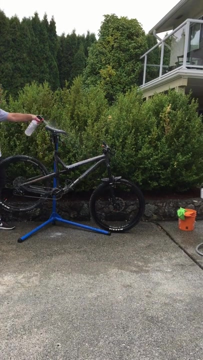 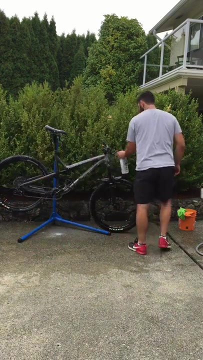 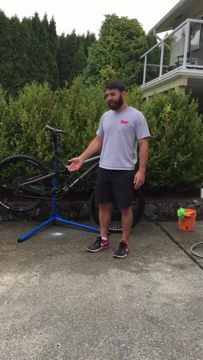 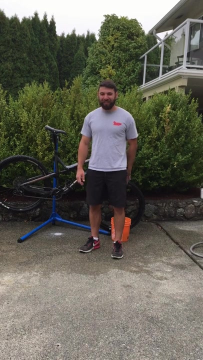 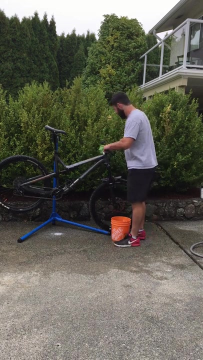 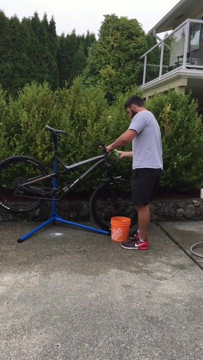 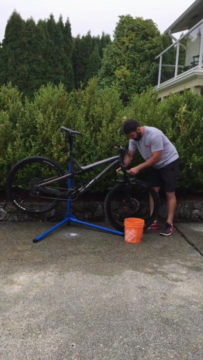 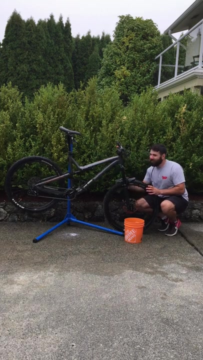 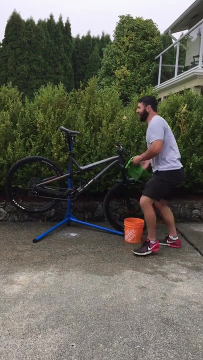 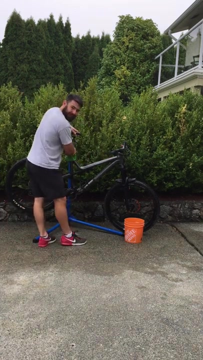 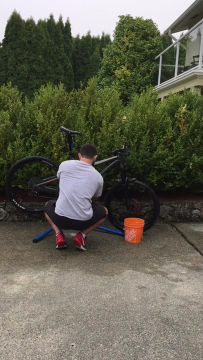 now that you've got your bike sprayed down, it's time to wait five minutes. let the cleaner do its work. so, now that it's been five minutes, grab a rag or a soft bristle brush and we'll give the whole bike a wipe down. it's time to clean up the rest of the bike. 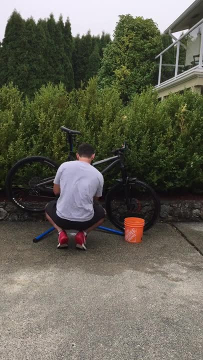 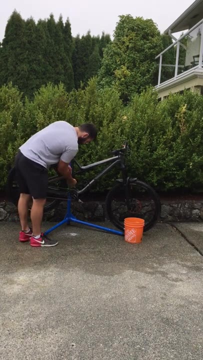 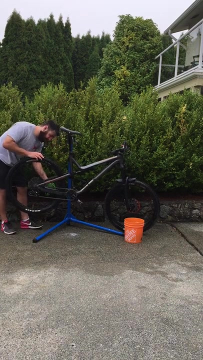 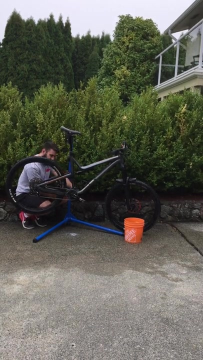 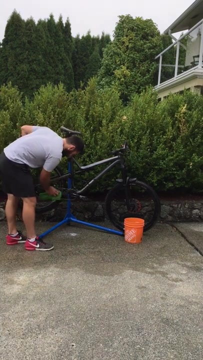 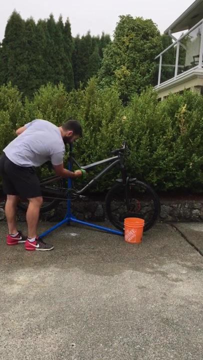 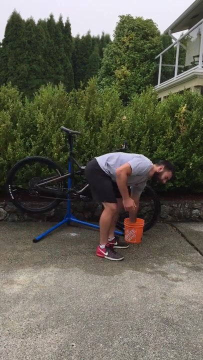 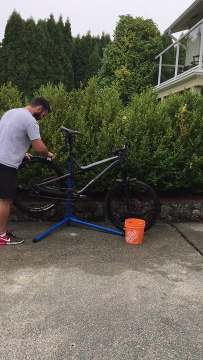 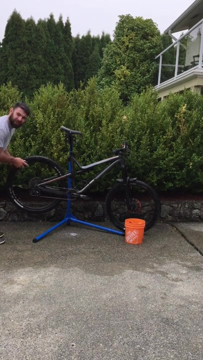 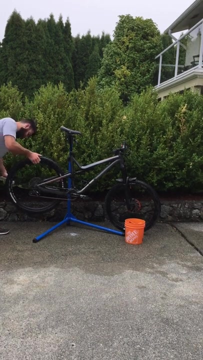 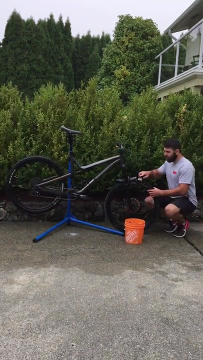 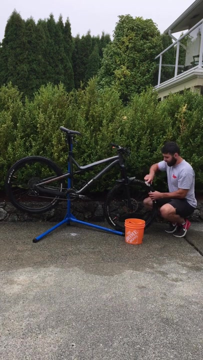 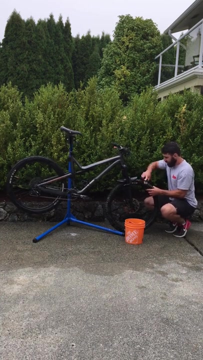 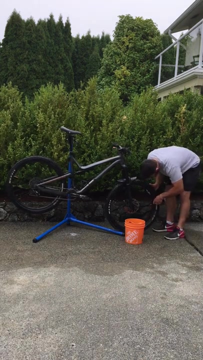 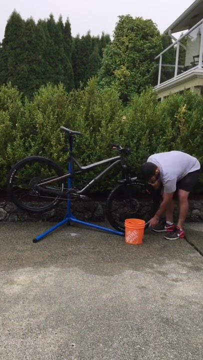 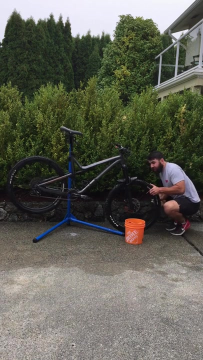 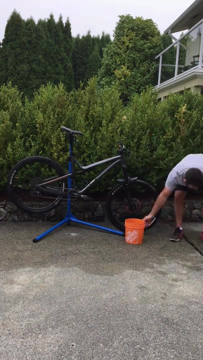 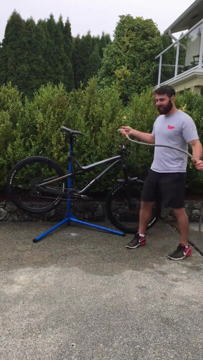 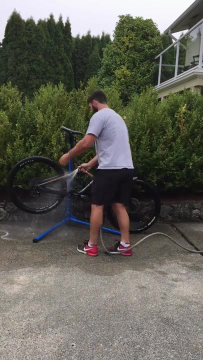 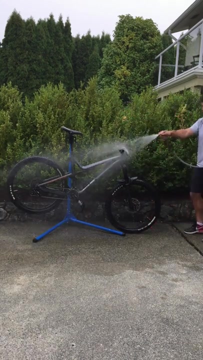 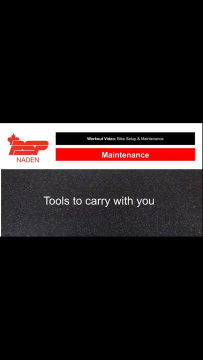 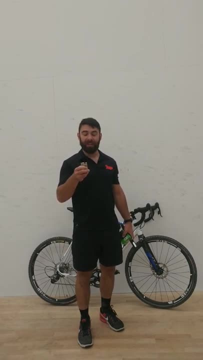 with you. i like to carry a multi-tool that has a few types of keys, screwdrivers and a chainring. also, i like to carry a stir tube, a pump and a 15 mil locomotive wrench- either a full chain wrench or a small chain wrench. of course, i just want to have a full size one or a stub. 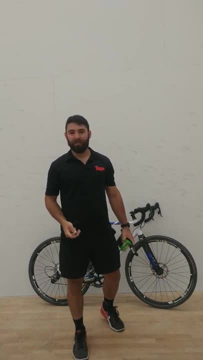 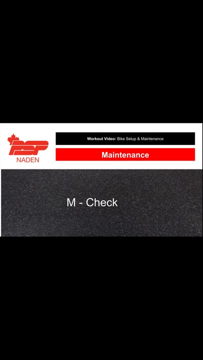 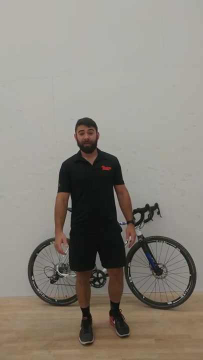 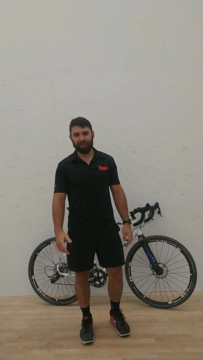 in the case of a mechanical vehicle, these simple things should get you back up and around. the rider can be tough on the bike, so it's always good to do a more thorough check every few days to make sure everything is safe. this is call them and what you're trying for. 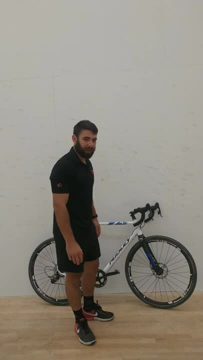 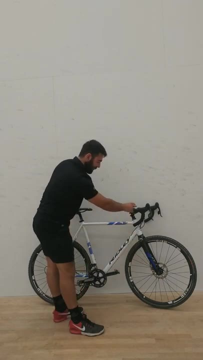 We're going to do a thorough check over the whole bike, making sure it's all safe To start. we're going to start at the front axle. move your weight up to the pedal bars, down to the body bracket, up to the seat and down to the rear axle. 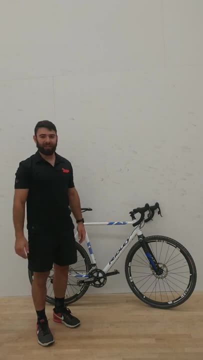 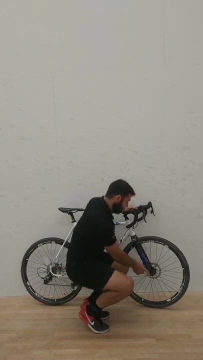 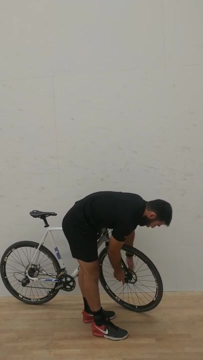 This creates an M-shape, hence why it's called the M-check. To start the M-check, we're going to start at the front axle. I want to make sure this is secure, so grab hold of the quick release, make sure that it's nice and tight and we'll come to a call. 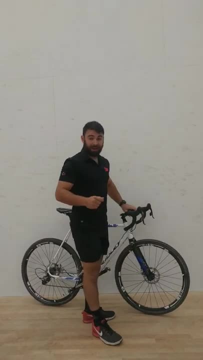 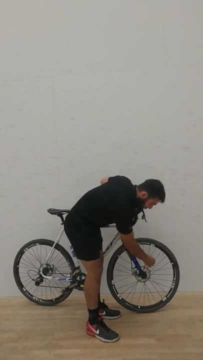 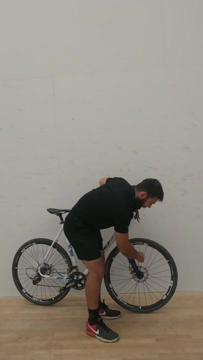 If you have a bolt or a nut holding it on, make sure that it's firmly on there. It's not going to fall off From there. you're going to feel each bolt squeeze into pairs together, making sure they're all nice and tight. 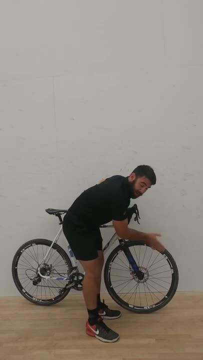 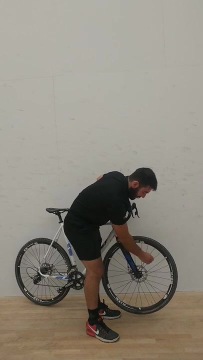 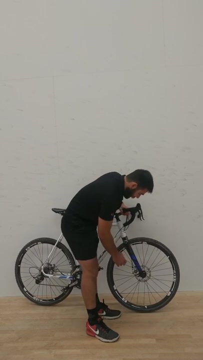 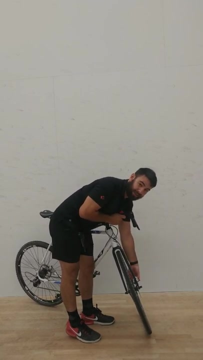 If you have any loose ones, this can unalign your rim, which is not good for riding. Make your way around a full wheel, making sure both sides are tight. Next, we want to make sure the brakes are secure as well. If you have good brakes, make sure the caliper is not loose at all. 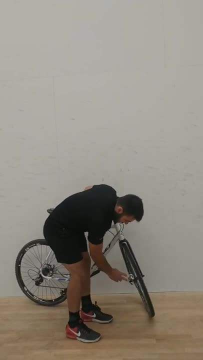 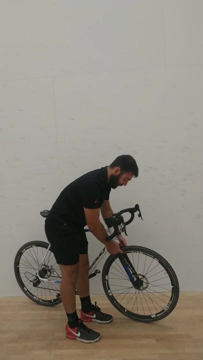 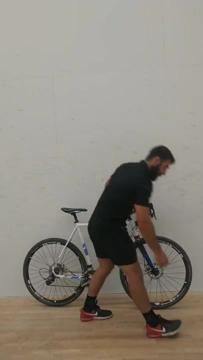 and, if it is, tighten up the back, two screws on the back of the caliper. Caliper, If you have rim brakes, you also want to check the bolts, make sure that they're secure. From there we'll move our way up to the stem of the handlebar. 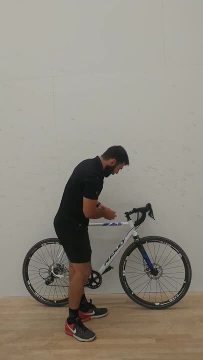 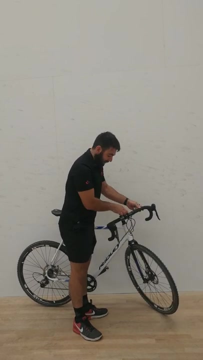 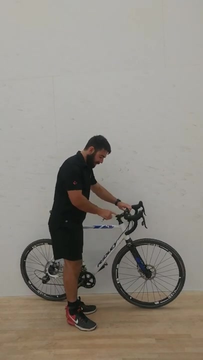 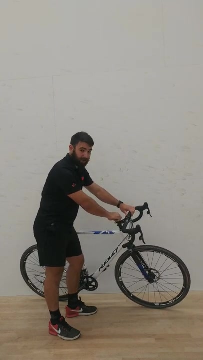 Grab a multi-tool, check each bolt on the stem, the top cap and the stem holding the handlebar into place. To tighten the bolt from the stem. we want to tighten the nut on the top cap first. They should be just snug and not over tight. 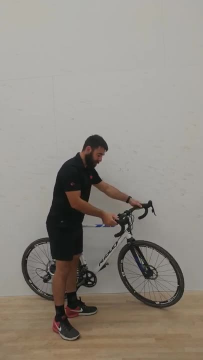 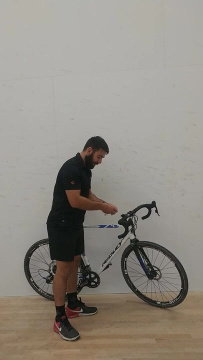 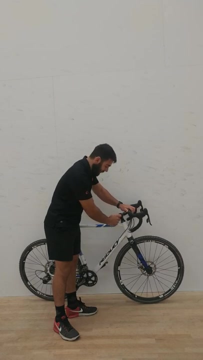 or else the handlebars will have a ratcheting feel to them, which will put extra pressure on the bearing. They're just lightly firm. Check that one first, then switch over and check the one holding the stem onto the bike. These should be nice and snug and tight. 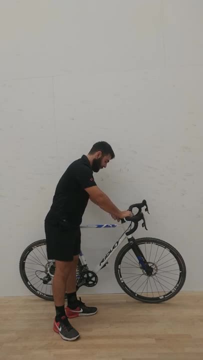 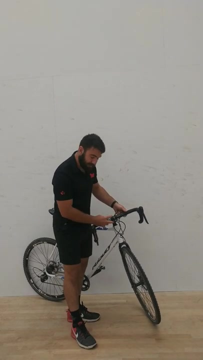 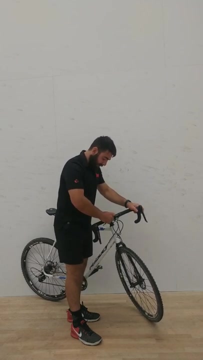 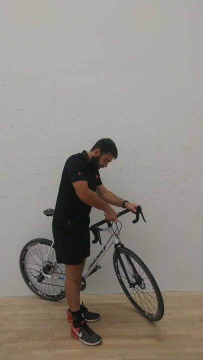 Give it a quick wrench, making sure those are tight. Next we can check the one that goes in front of the stem, Which one holds the handlebar in place. To do this, start in one corner. If you have four bolts, give each one a tight trough forward to the opposite corner. 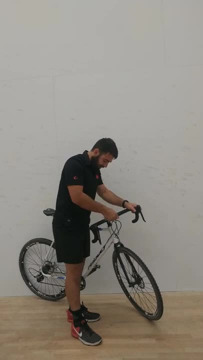 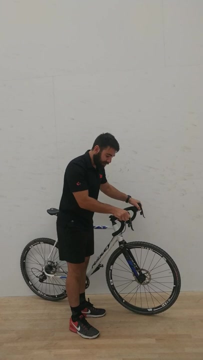 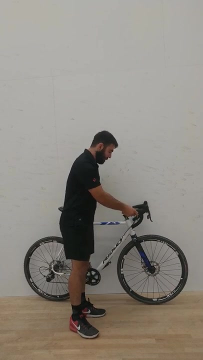 and up. And finally the last one: These should be fairly snug. We don't want the handlebars moving at all. Next, you can make sure your brake levers are secure and shifters are secure in there. Tighten them as necessary. 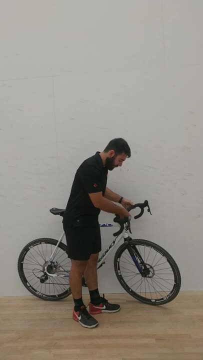 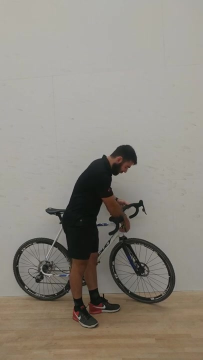 You can check on the handlebars. The final thing: you want to take a look at all the cable housings. Make sure that they look nice and they know what types of wear are. Once you've done that, we're going to move our way down. 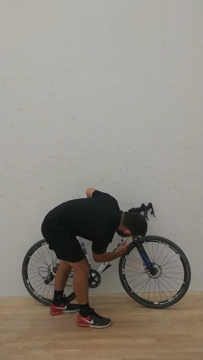 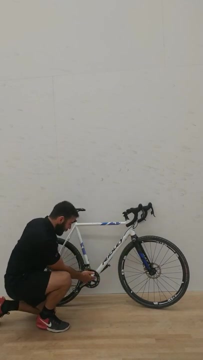 The bottom down tube of the bike. Make sure there's no wear or tracks in the frame at all. Check all underneath And we'll get down to the bottom rack. With this. we want to look over all of the gears in our chainring. 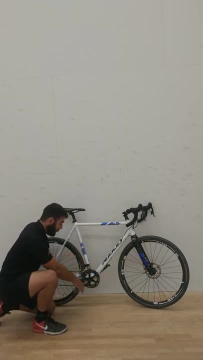 Make sure there's no wear or bent teeth. You can go all the way around. Make sure that's all good. Tighten it If you have a front derailleur. make sure that's six-seater in place. Next we can check our pedals. 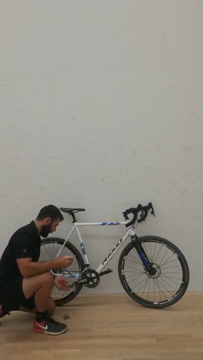 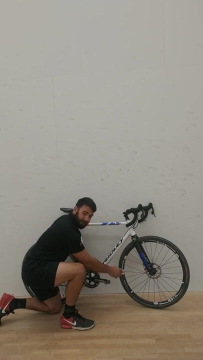 Let's see where those 15 mil Oakman and Wrench come into play. Check the pedals. We'll start on the right side, The right one, a regular ceramic pedal. So bring your pedal to the front position, Place the wrench towards the front wheel and press down. 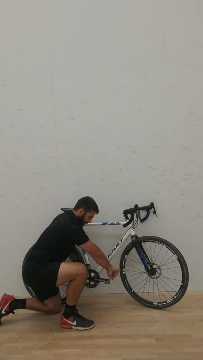 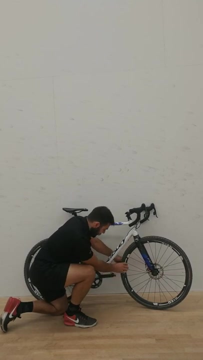 This should be nice and tight. Tighten that up nicely. Then switch to the other side. Now the left pedal is reverse threaded, So we're going to do basically the same thing. Pedal is out front, Put your wrench towards the front wheel and also press down. 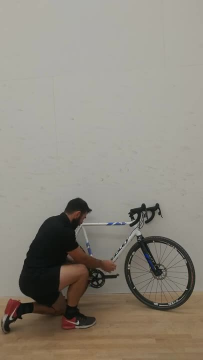 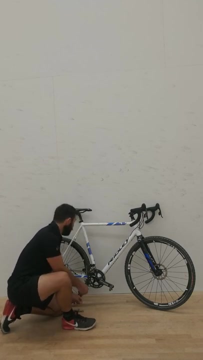 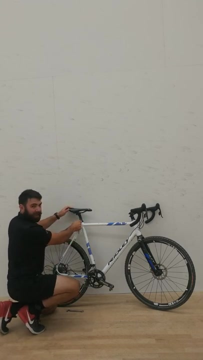 Make sure that one is tight. Once that's good, you're ready to move on up towards the seat. Make sure. if you have a bolt securing your seat, make sure that's nice and tight. If you have a quick release, make sure that's tight. 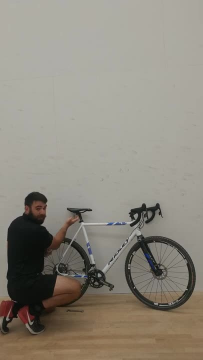 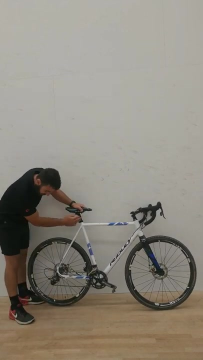 You don't want the seat moving up or down. Next, you can check the bolts underneath the seat. Make sure those are secured well. Finally, from there we're going to move down to the rear axle. Again, we're going to check all the bolts on our rear wheel. 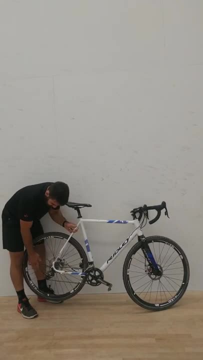 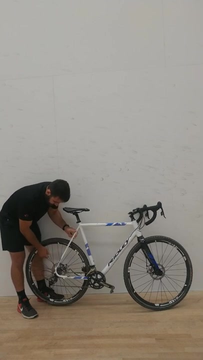 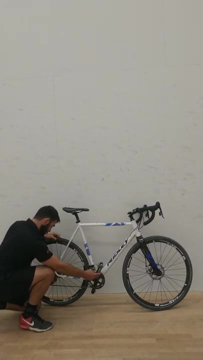 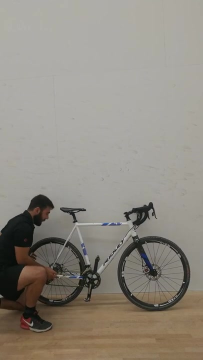 Make sure those are all nice and tight. Make sure you check both dots. Next we'll take a look at our rear cassette, Making sure that there are no bent or broken teeth. Go all the way around checking each gear. Next we're going to check the rear axle. 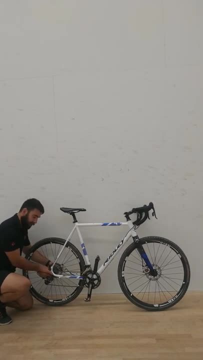 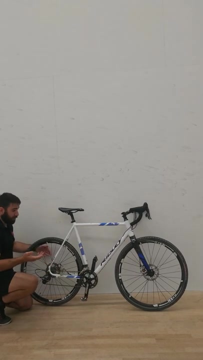 Make sure that's nice and secure and nice and tight. We don't want this follow-up or shifting around on us which will cause unnecessary wear or possibly a crash. Make sure that's nice and tight. Check the cable leading to the rear derailleur. 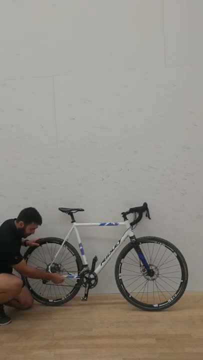 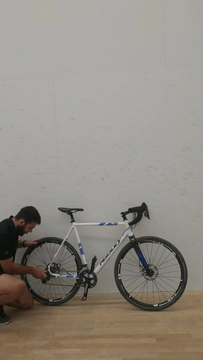 Make sure that's in good working order and not worn. Check to make sure your derailleur is secured to the bike. Sometimes with the rattling or driving that can come loose. Grab your mower tool again and just double check to make sure that's secure. 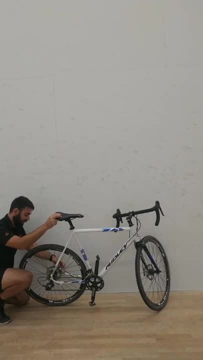 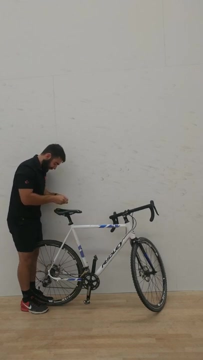 Finally, we're going to look on the left side for the brakes. Again, we want to make sure this is secure to the bike, So check both bolts, Make sure that they're tight And if you have rim brakes, check those as well.